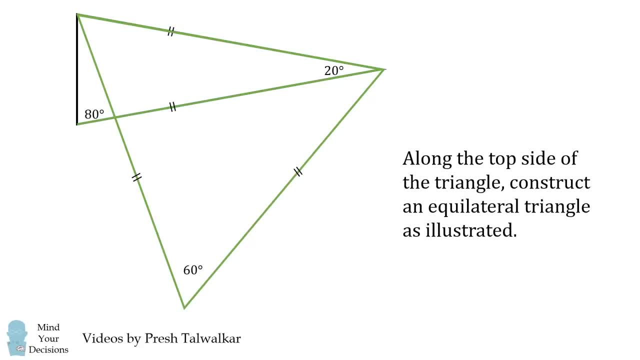 So this is 60 degrees. this other angle will be 60 degrees in total, so this will be 40 degrees, and here we have another 60 degree angle. since the very top angle is 80 degrees, we know that this will be 80 minus 60. 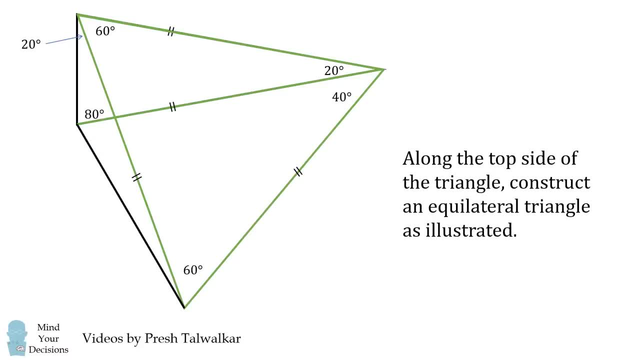 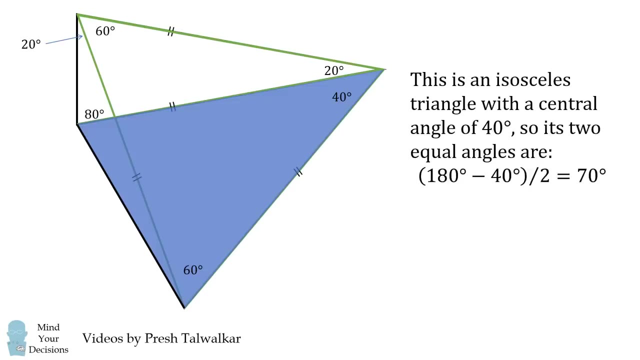 which is 20 degrees. now let's connect these two points and, furthermore, we'll focus on this triangle. now two of the side lengths are equal to each other because they both have the same length as a green side, so this is an isosceles triangle with a central angle of 40 degrees. 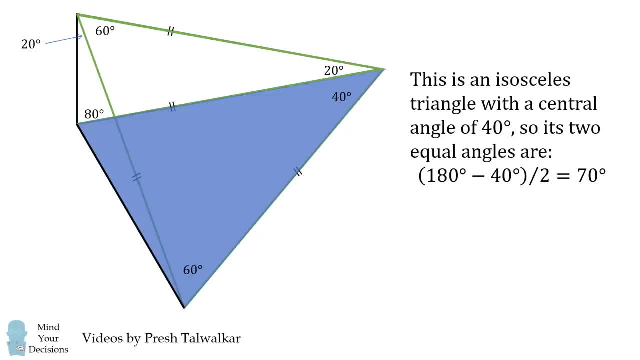 which means its other two equal angles are 180 minus 40, which equals 140 divided by 2, which is 70 degrees. so here we have a 70 degree angle, and the other angle is also equal to 70 degrees. so if we remove 60 degrees from it, this will be equal to 10 degrees. 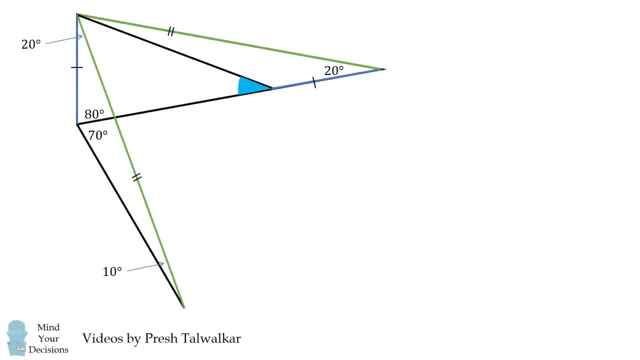 now let's go back to this diagram and we want to solve for this angle, and we want to solve for this angle, and we want to solve for this angle over here. how can we do that? well, here's the other insight. look at these two triangles now. they will be congruent to each other by side, angle side, because both of these triangles have. 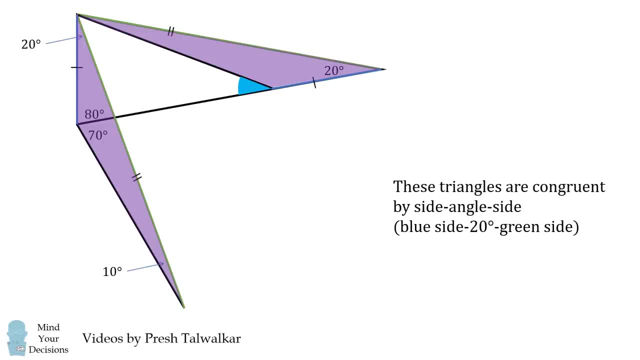 a blue side, then a 20 degree angle and then a green side. this means there are obtuse angles will be equal to each other. so this angle here will be equal to 80 degrees plus 70 degrees, which is a hundred and fifty degrees. finally, we can solve for the angle that 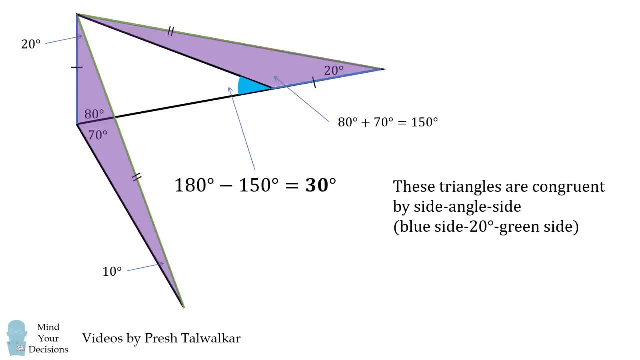 we want, because this angle is an obstruction. so we want to solve for the angle that is want to. This will be equal to 180 minus 150, which is 30 degrees. And that's it. Did you figure it out? Thanks for watching this video, These math videos. 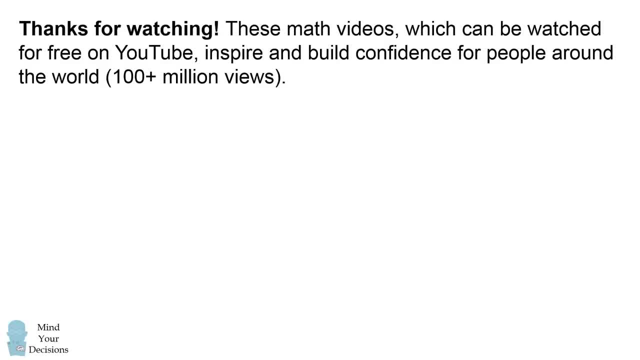 which can be watched for free on YouTube, inspire and build confidence for people around the world, and they have over a hundred million views. Please subscribe for free to get the news videos and you can email me a puzzle or math topic presh at mindyourdecisionscom, If you so choose. you can check out my 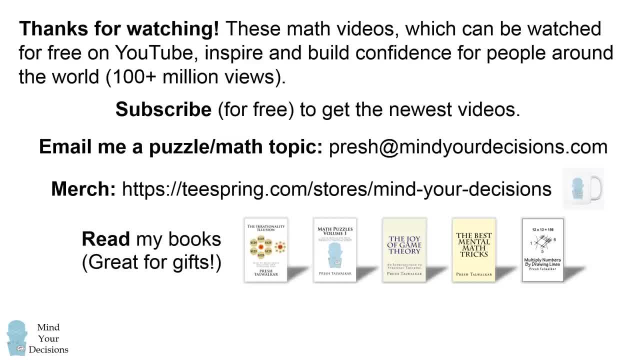 merchandise which is listed on Teespring. You can get my books which are listed in the video description, and you can support me on Patreon for exclusive rewards. Thanks for watching and thanks for your support.